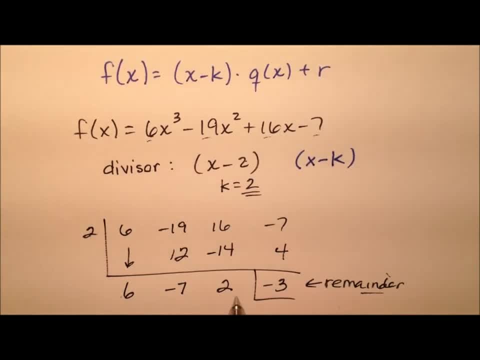 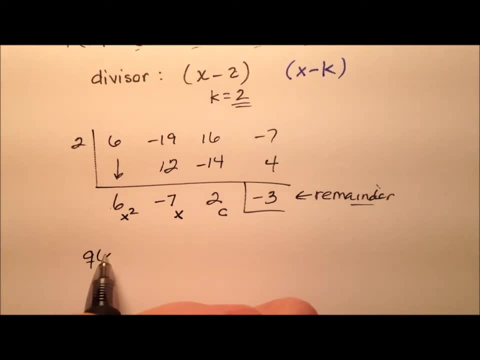 negative 3.. Okay, so, when I build this back up, here's my constant, my linear term and my quadratic term. So my q of x, which is my quadratic term, So my q of x, which is my quotient, ends up being 6x squared minus 7x plus 2, and my remainder then is negative 3 and my 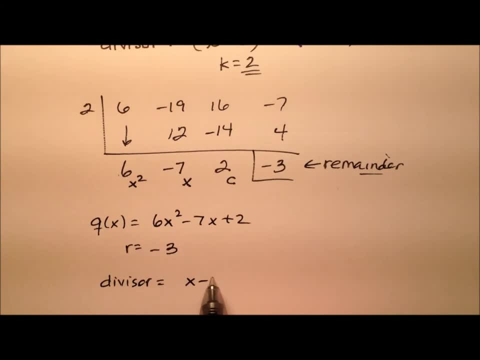 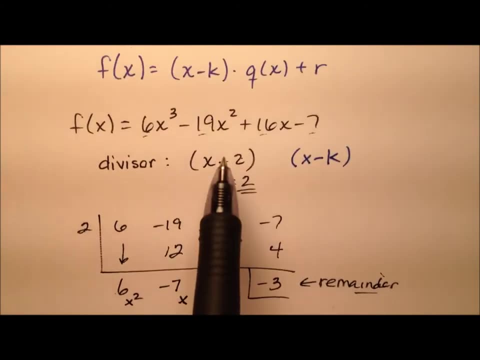 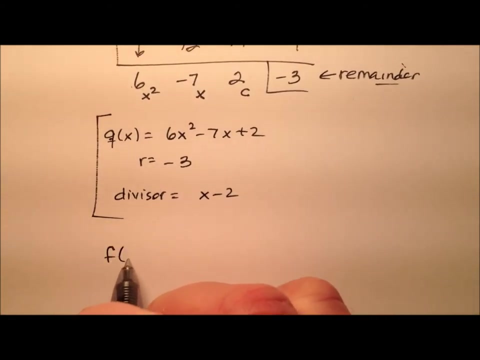 divisor that I used at the beginning was that x minus 2.. Okay, so now that we have all three pieces, the q of x, the r and the divisor, I can go ahead and write it in this form. Okay, so I'm going to say my function can be rewritten as: 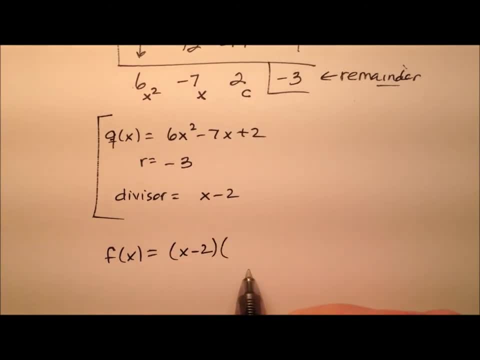 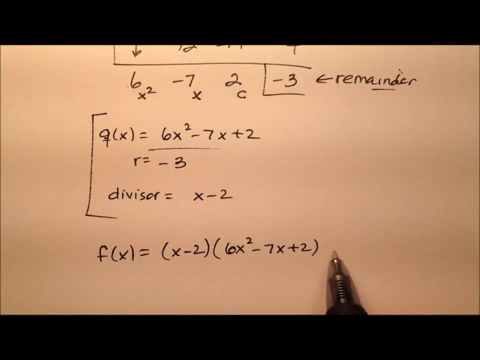 the x minus 2, which was my divisor times my q of x, which is this quotient polynomial here, this function, and then plus and it's a negative right here. so sometimes I've seen a plus, a negative 3 in parentheses or just a minus 3.. I think for now let's go ahead and put plus a negative 3 and have. 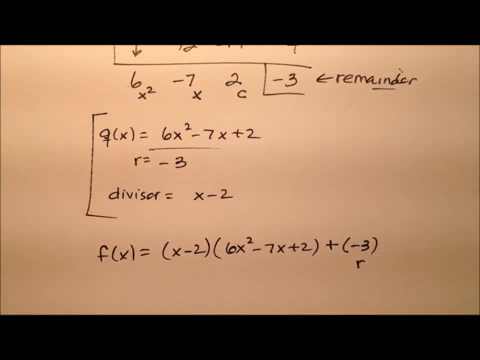 the understanding. that's my r value, and you can just as easily just say minus 3, and that's okay too. So here's my divisor, And then here's this q of x. Okay, so why do we write it in that form? Well, a couple of reasons. 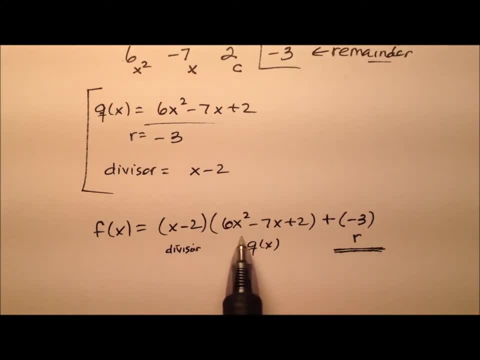 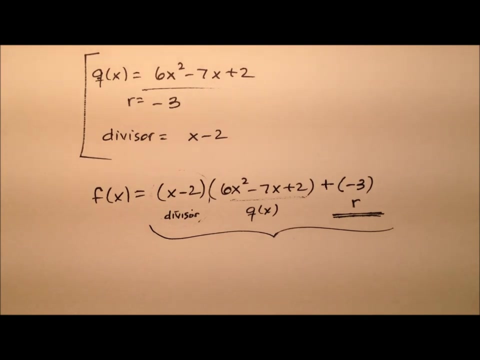 One, so we can see what the remainder is, and so we can kind of differentiate between the quotient and see just if this divisor, what this relationship is when I divide this polynomial. Okay, so let's go ahead and multiply all this back out and I'm going to show you that we should end up with our f of x. 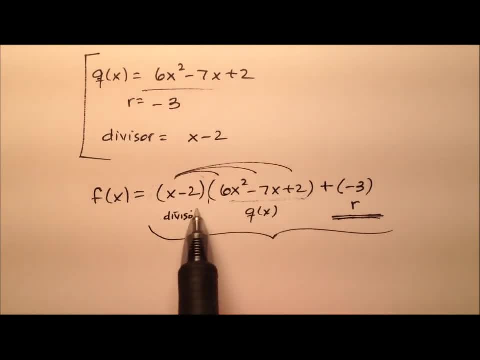 once again. So we'll go ahead and distribute through this x and then this negative 2, and then, when I'm done, I'll add this negative 3 which was our remainder. So x times these terms will give me 6x, cubed minus 7x, squared plus 2x, and then, when I multiply by the 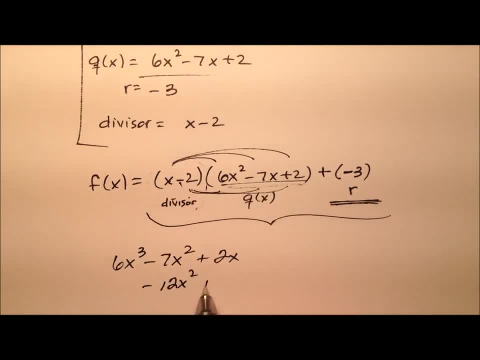 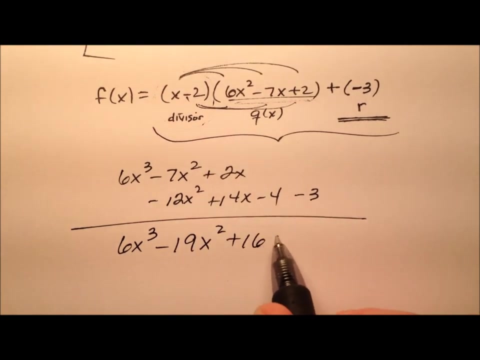 negative 2, I'll have negative 12x squared plus 14x, minus 4, and then there are a remainder here of negative 3. So I'll kind of just put it all together. So you get negative 5x cubed minus 19x squared plus 16x minus. it looks like minus 7..